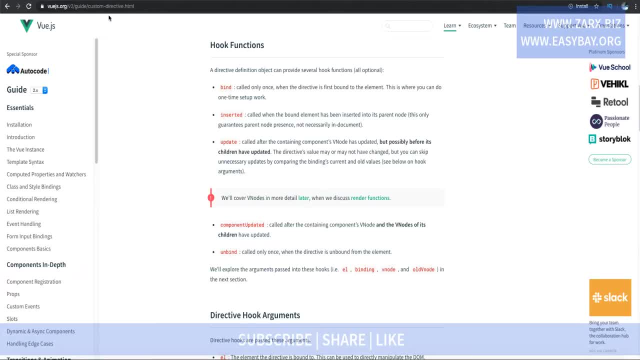 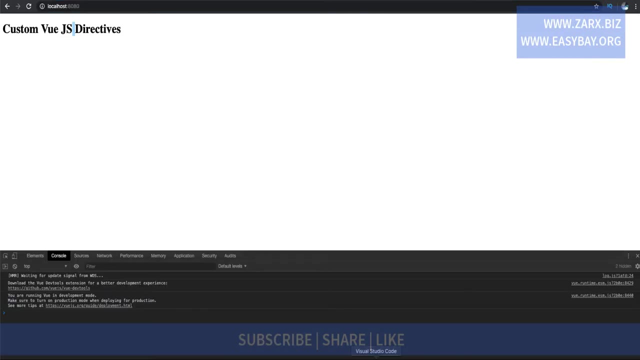 we do using Vue hooks for custom directives. if you go into the custom directive documentation of Vuejs you will find here hook functions. they are bind, inserted, update. now what we are going to do. we are going to see first of all the bind one. so to working with the bind, we just call it bind. 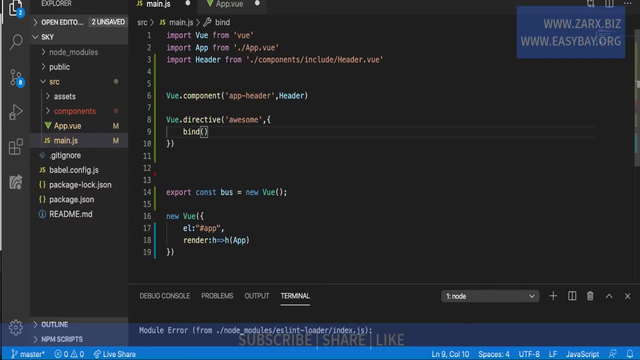 and we get few parameters arguments here. first is element and the second one is binding and the third one is v. note now: if we be using them, we are going to, we can pass them here. if we are not using them, you can remove them. you can use only two as well. so what exactly these? 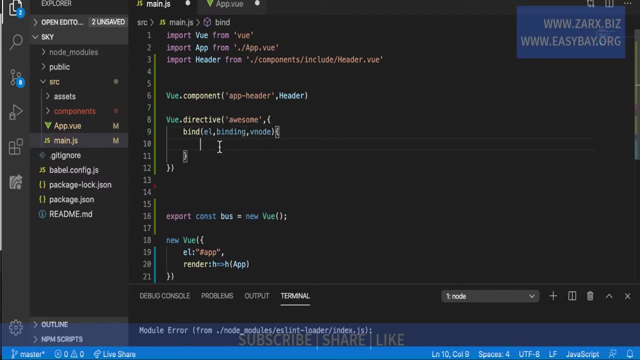 are. what happens is- this is a kind of function- first is element. so wherever you're going to include your directive- just for example, we included this view beyond or this edge one- so if you'll be using your custom directive on this one, it is going to match this element and it is going to. we can chain that element using this r. 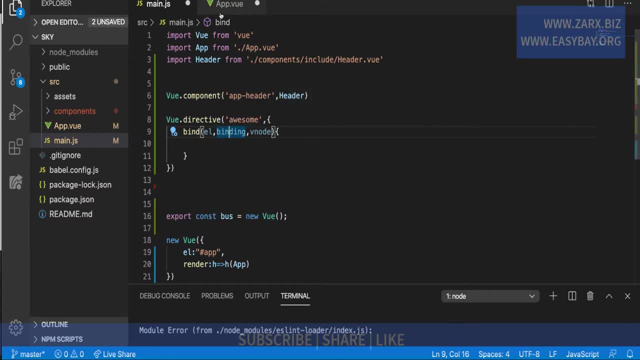 now the binding is going to get the values. so when you pass a value inside it, let me show you. so what we do here is we already have it. so we have awesome directory we just created. i saved this file. go to appvue and remove this code and call our custom directive. so i'll say v awesome instead of on, so this is how you call it. 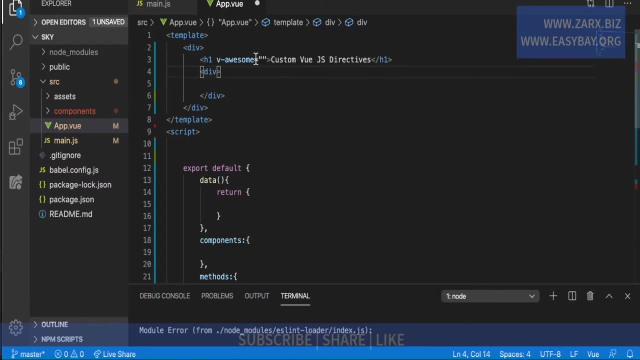 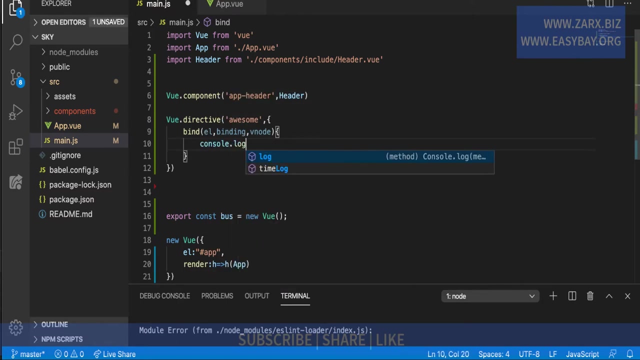 and when you put here anything you're going to put, it is going to be the value, and that value we can catch using binding. so if i say let's put a string in here, so i say something: all right, so let's save this, and i go here now we can catch this. so we say console dot log. 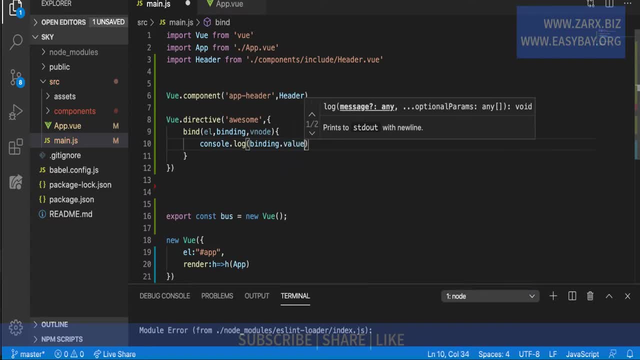 binding dot. well, so this is how we use the value now. the third one is v node. it's a virtual load. we are not going to use it much in professional projects. you will use this very rare, mainly be having to work with the element and the binding. we will talk about original later, but for now we have this. 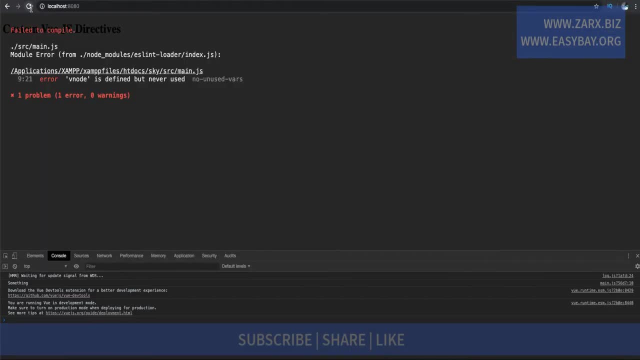 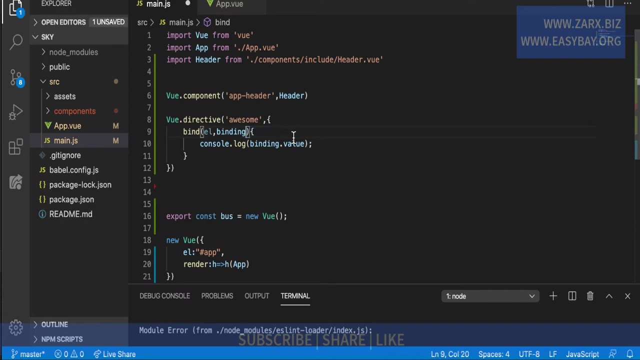 binding going on. now let's see the browser. we have uh error. it says v node is defined but never used. so we defined it here but never used it. so let's remove it because we are not going to use it for now. so if i go there we get custom vgs directive, which is uh the this line. so we need to check the. 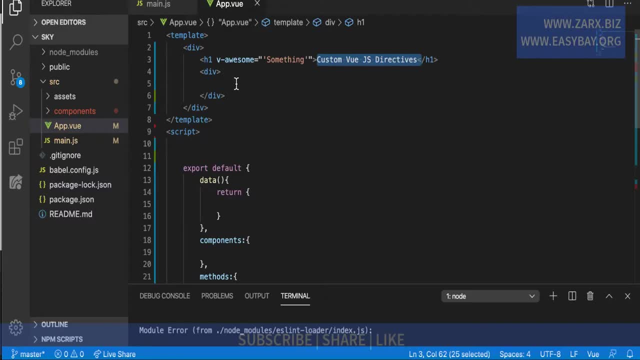 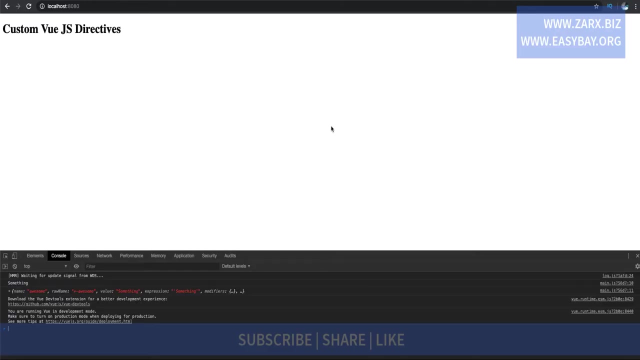 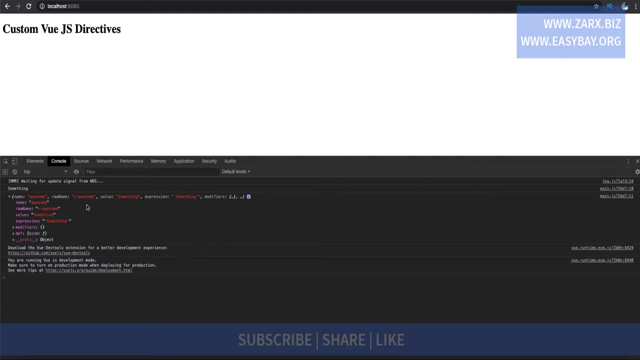 console and we have something in there. so there's something that we are saying here: now binding has so many things in there, so many elements, so you can check that as well. so if i copy this and i remove this value element and we can go and see that now we get name: awesome, so it is the directive's name, and then we have the. 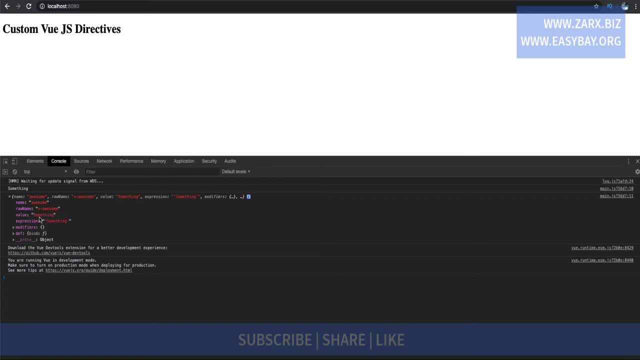 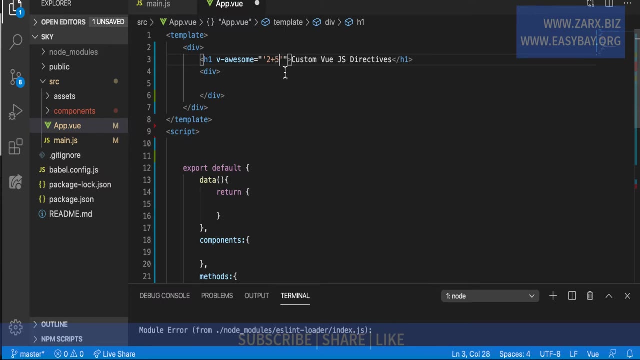 full name of directory: raw name. we have value, we have an expression, so we can get the value as well as expression. let me show you the difference between these two. so just for uh example, instead of uh something, if you say two plus five here and you save this, and then you can. 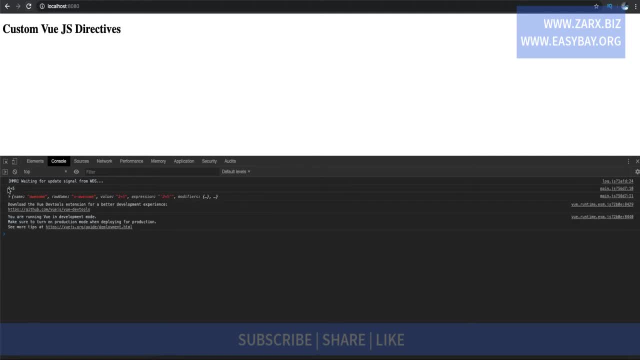 when you go to and refresh the page, you get two plus five. uh, i mean, remove the string, because this is passing as a string right now. and, uh, we get seven. you can see here now: uh, if, and this is the value, we're getting seven. so it is calculating the value and giving us, but if we go to expression, 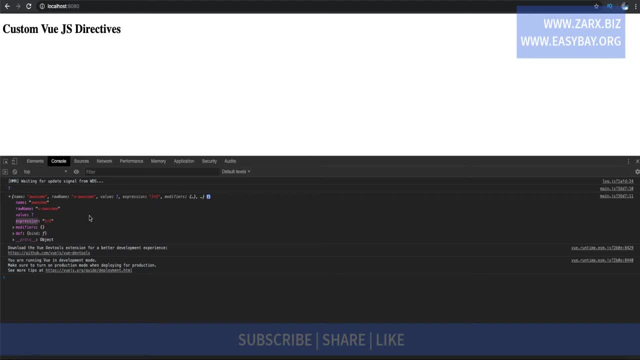 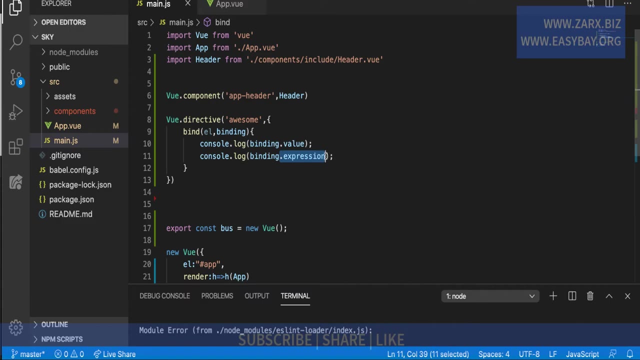 we get the? what exactly thing we are passing? so, instead of passing value, if, uh, you say here dot expression, so we are not going to get the seven, we are going to get two plus seven, uh, two plus five. so this is the difference there now, if we remove it again and go there. so what are the? 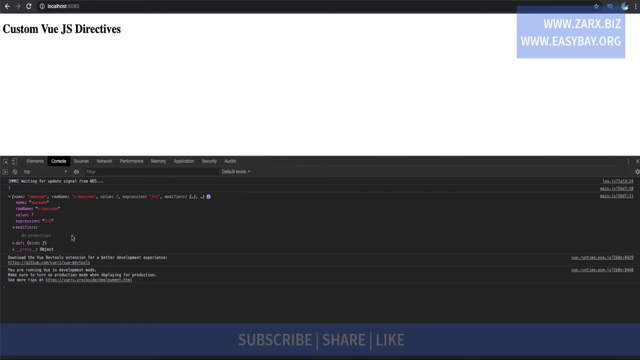 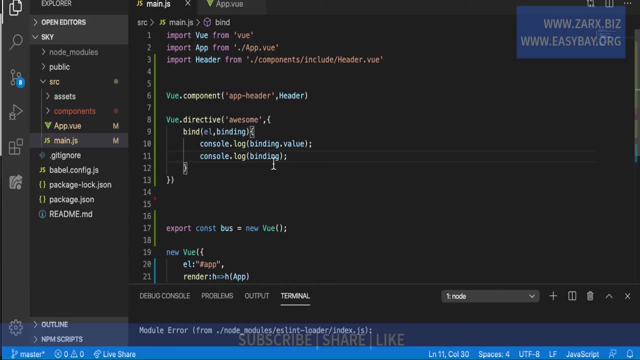 other values we are getting. we are getting modifiers personally. uh, no properties there. we need to see that in a moment. so, uh, let's play with some data here. so what i do? i am already getting the value. i want to use the element tag as well. so so we can do. 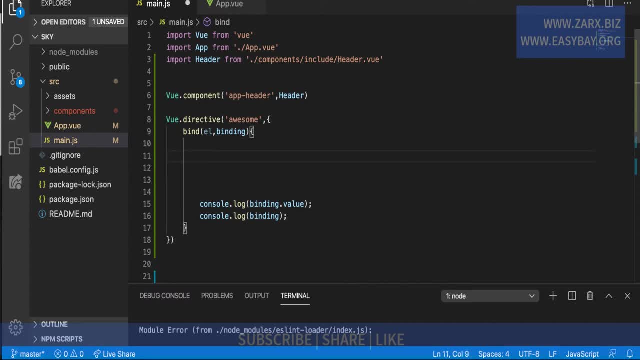 this way we can say this element that i want to change the text here first of all, so i can get the element using l, because we called it here and i say element dot, and to work with it. you can use it like javascript whenever javascript. so we say inner html. 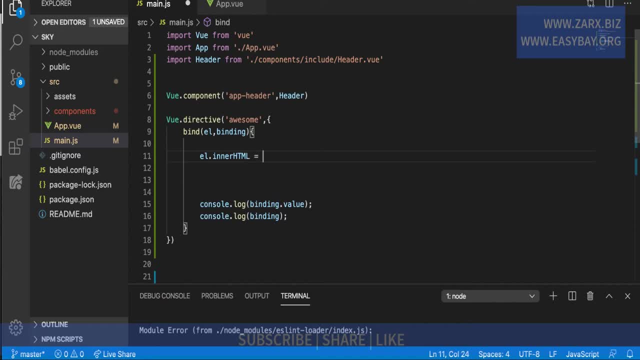 and uh, we're going to say here if we want to pause and let's say we are passing the value, that we are finding that value, okay, so let's save this, we get seven, let's put some value through the property. so i say tagline view js custom directives. 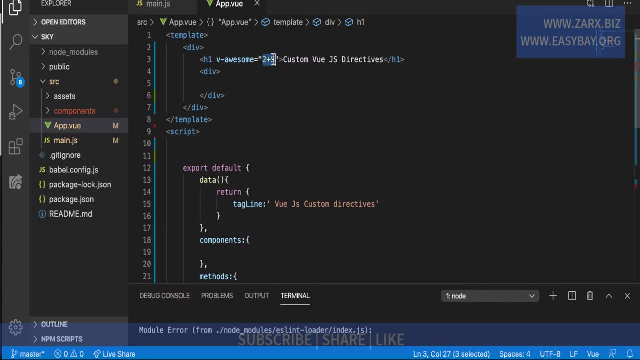 and we pass this in here, all right. so now, very fresh, we get vgs, custom, uh, the string that we saved here. now we can play with the content as we want. we can even say that element, dot style, dot color. so you get the idea. mainly, what i'm doing here is i'm just treating this as a 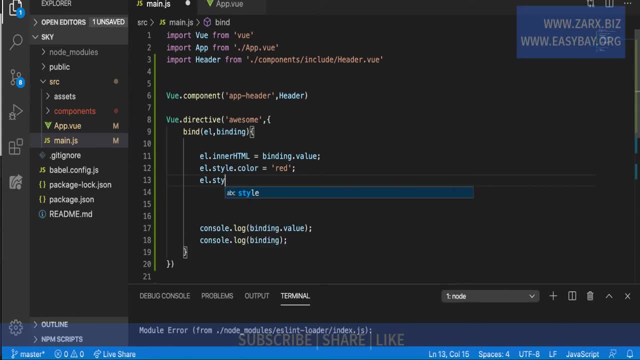 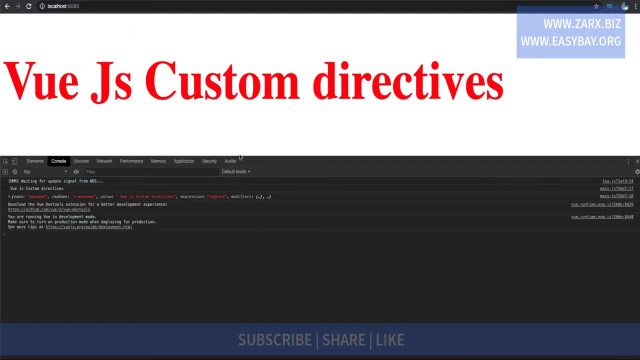 javascript so you can do anything that you do in javascript. so size and you can say here for your pixel: so if i save this, we have it red, we have it big, let's make it more big. so you can see that in we directives we can pass arguments in custom directives. so if i say here common and then i say 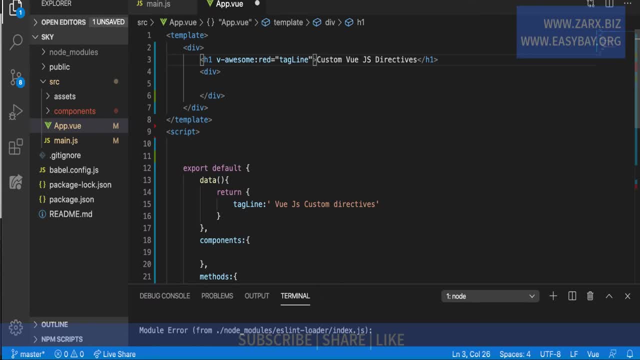 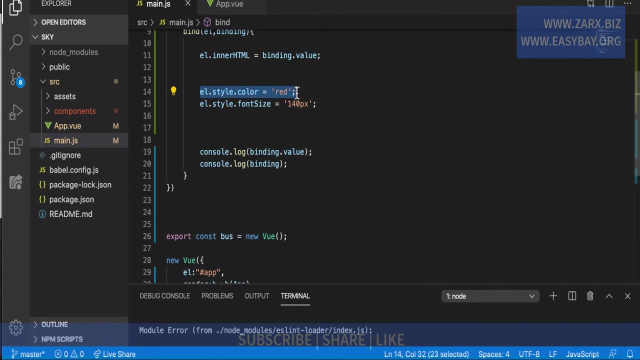 now. previously we just used arguments so we can put in an argument format and then the argument is now. previously we said red here as a color. we just passed a string here so we can pass the value from here. so if i save this and if i go here i can put a condition to change the color. 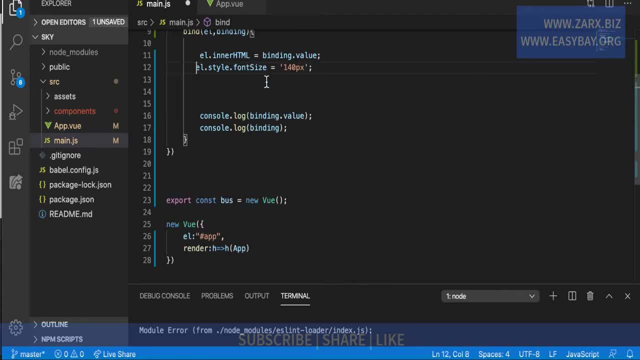 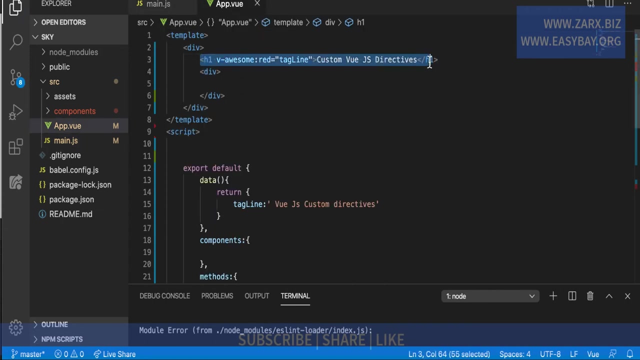 let's do that. so i just put this with that one. and here i say: if binding and dot arg is equal to red, then do this, else do this so we can say: here green, now we have here red. let's copy this line and put in here instead of red. so i'm going to put a green here, so you. 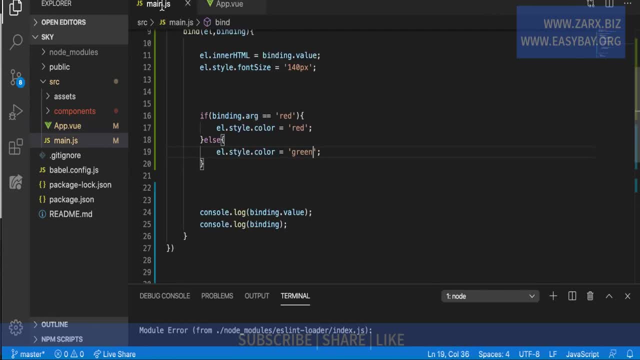 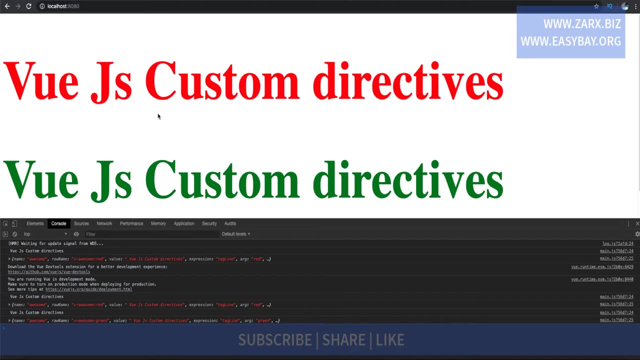 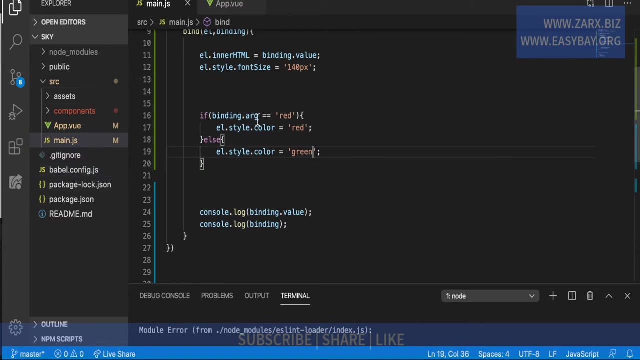 can see that this time we have positive red here. green, it will check. if it's the argument's red, it will turn it to red, otherwise it will turn it to green. so if i go there, we have vjs custom directive in red and in green. so this is how the arguments we can use in custom directive, but that is not a limit. 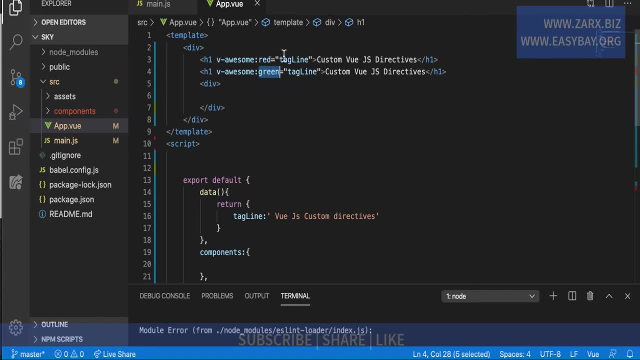 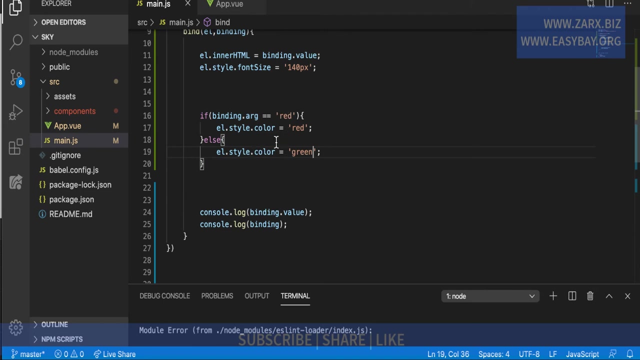 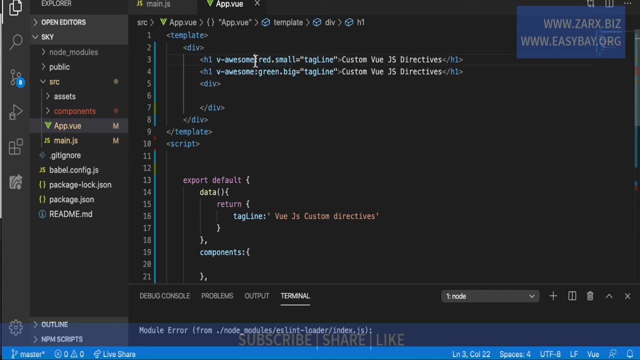 we can even add more arguments in this one too. so what you add, let's say small in here and big in here. so in this case, all we we'll be using the same thing but a little differently, because it is going to be a modifier thing that we are going to do so, to do that. and now we passed here to and we need to put dot in. 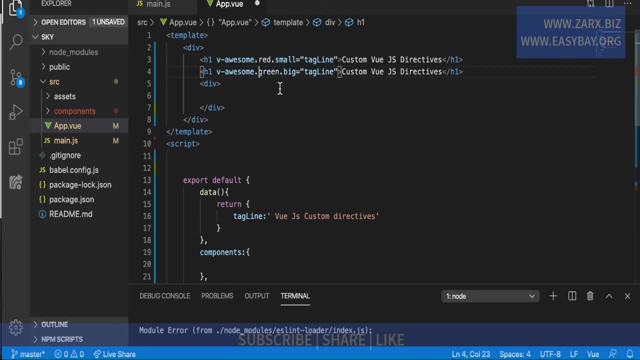 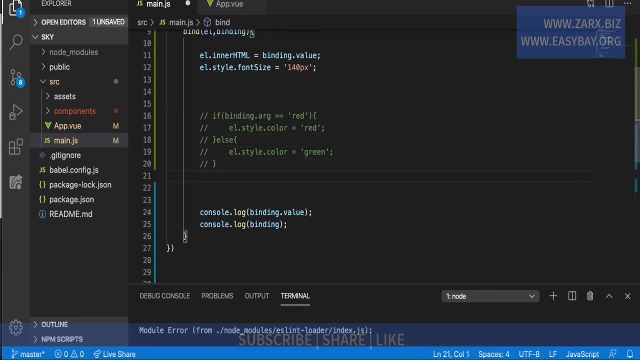 here. so this is going to be this way: now, when you go to the mainjs, where you, first of all, are in need to command this, and this time, when we are going to check for it, we are going to check something like this. so we're going to say: element dot, style dot. 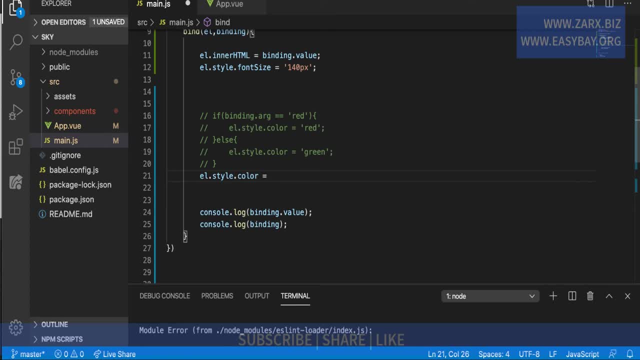 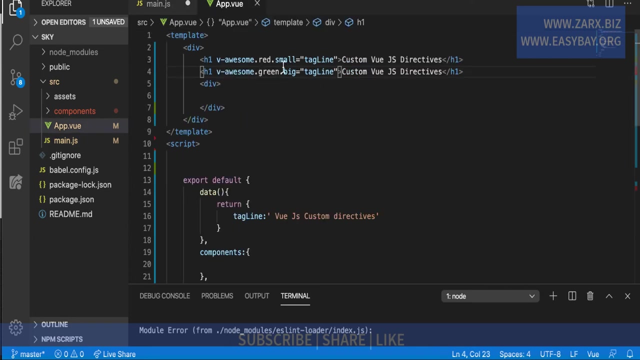 color and equal to binding dot modifier modifiers dot red, because we provided it. if it is red then it is red, else let's make it blue, it's going to be string and similarly we provided. the second thing is small, red and small, so we can say: 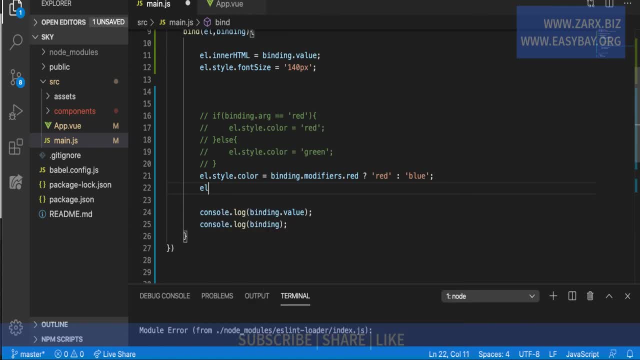 here: element dot: style: small. if this is the case, make it 40 pixel, 14 pixel. otherwise make it 50 pixel. so this is a ternary operator. we check. if this is valid, then do this. otherwise do this. so this is how you do write it down. it's just something like: 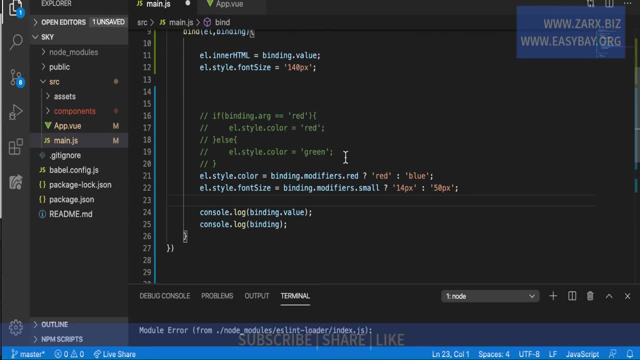 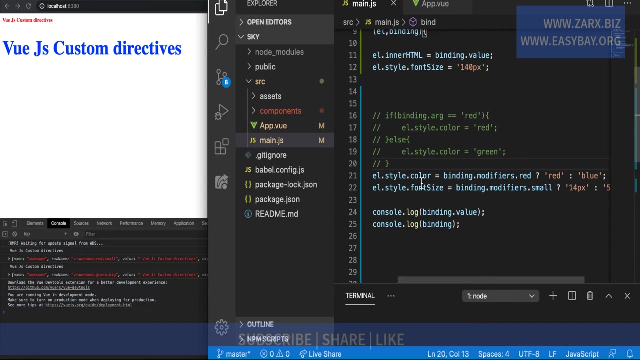 if condition, if you've never seen this before. so if I go to, I need to save this file and if I go to, here we get. let me take the code here. so we mentioned here that if the modifier is red, then make it red, and that is red there and not red because the other one is not red. it's. 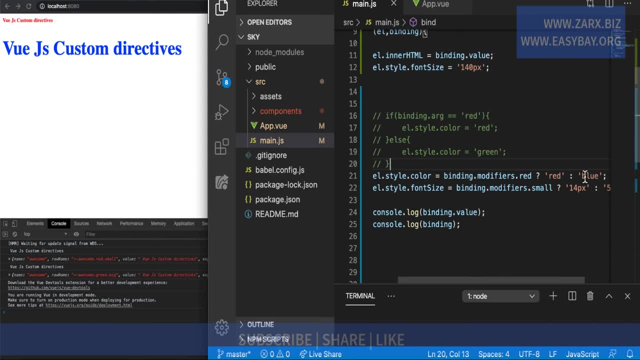 green, so it is checking that it is not red and it's just doing it blue. it turned it to blue. similarly, it worked on the font size and it checked the small. where the small is applied, we applied the small on this one and big on this one, so where it was small, it added 14. 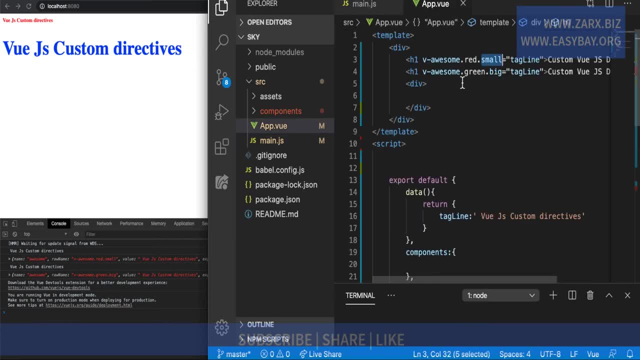 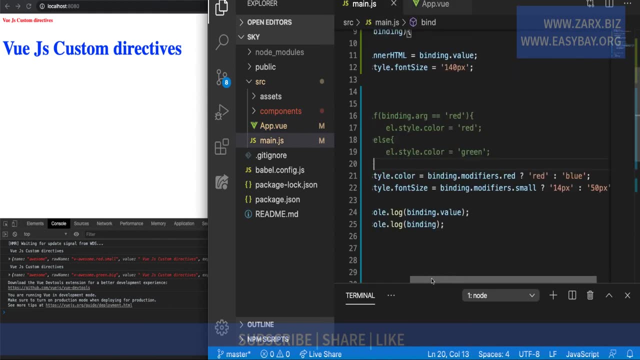 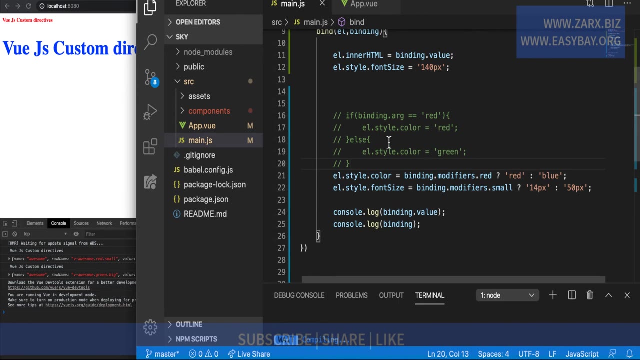 pixel and 50 pixel where it was not small. so if you say big you can write another condition. but we used ternary operator to make it work this way. so now you use modifiers with the custom directives and you can do any kind of operation with this. so so far, so good. we work with the arguments as well as. 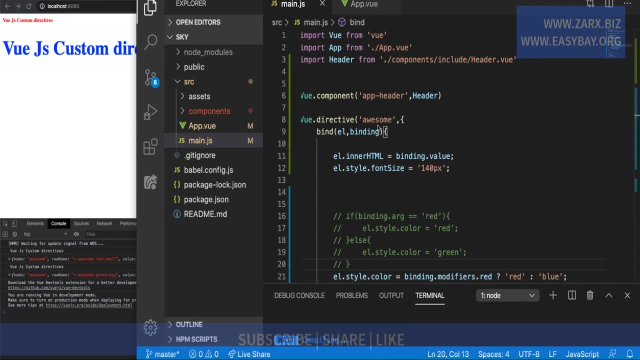 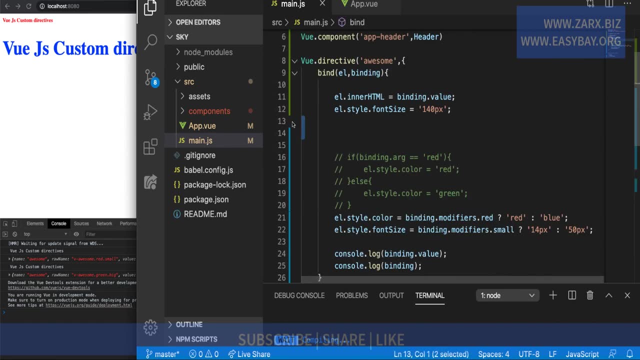 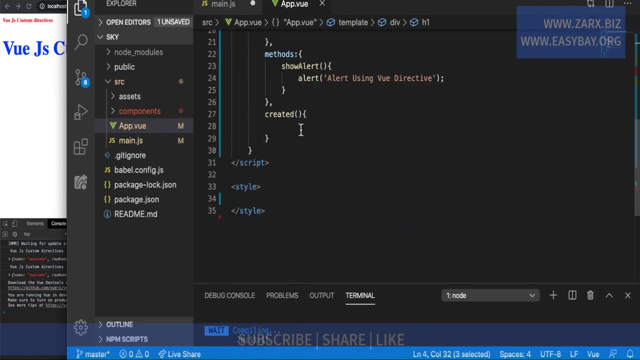 modifier. we define this directive- awesome directive- globally, so now I'm going to show you how to define it locally. so, to define it locally, what we need to do, we need to go into our view component, wherever you want to define it, and it is just going to be one of the, just like these components and methods. 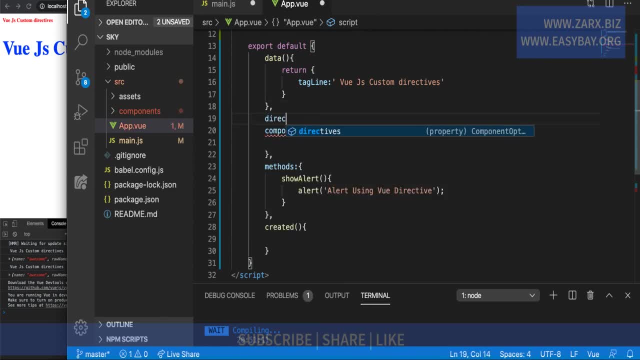 we need to include it here. we just say directives and just similar syntax, so inside it we can define our directive. so we created the directive with the name of awesome. so I will put here, and when I put the awesome it's going to be something like this and that's it. we just created the awesome directive.